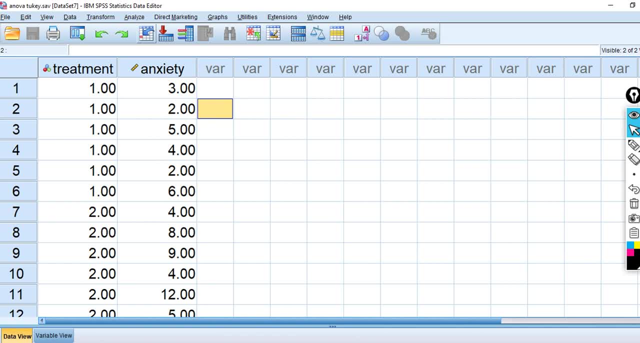 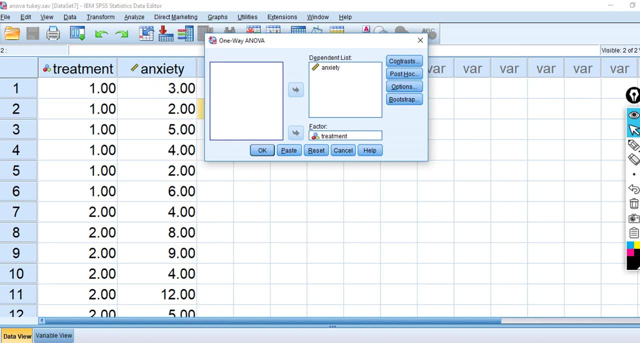 essentially this involves comparison of means. So we're going to use this just as a point of comparison. So let's go to analyze, compare means. one-way ANOVA and you see that I have the independent variable treatment in the factor box in my dependent variable anxiety and the dependent list I've also clicked on under options. 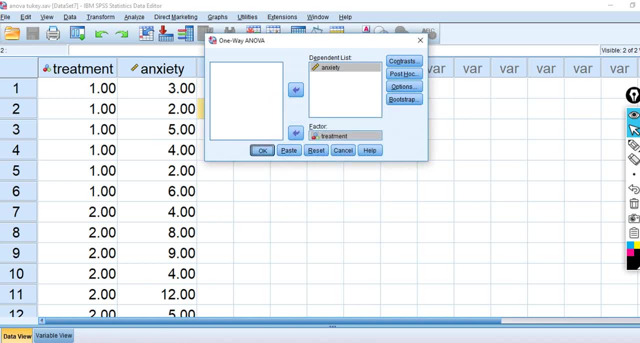 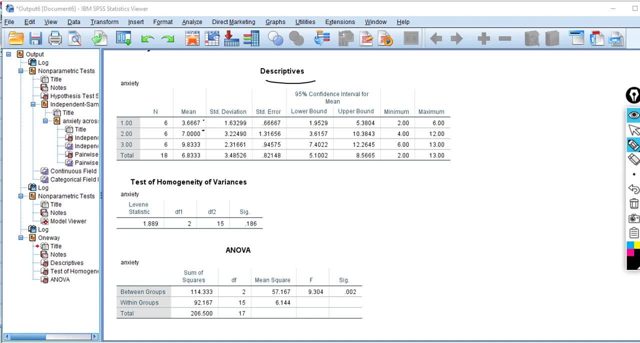 descriptives and homogeneity of variance tests. So running this analysis you can see that we have under descriptives we have the means for each of the three groups. So you can see that the mean for group 1 is 3.6667,, the mean for group 2 is 7, the mean for group 3 is 9.833.. And so essentially the 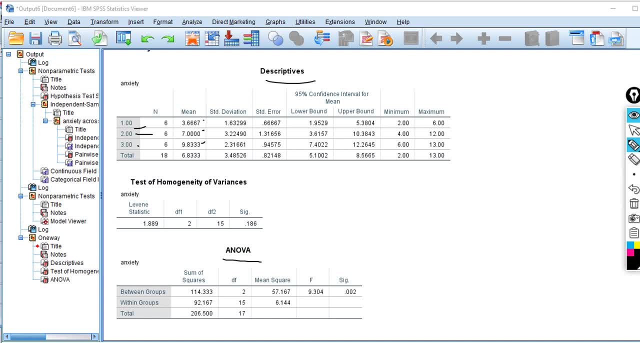 one-way ANOVA is involving and is a test which helps us to draw an inference about the population means on our dependent variable And essentially, if our ANOVA results are significant, then we would infer that there are significant population means across the groups. 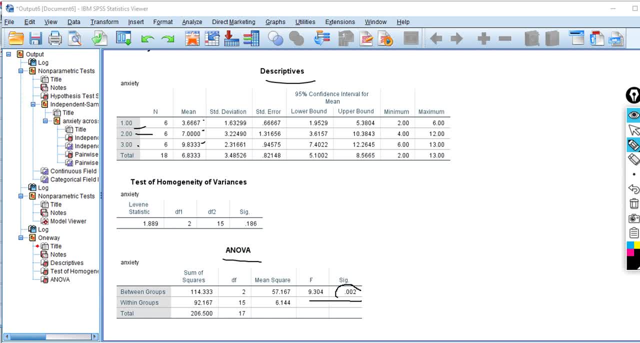 So you can see, right here we have the F test and our p-value- that's printed out right here- which is point 0.002 less than conventional point 0.05 level. so we would essentially reject the null that the population means are all equal and infer that there are differences among the population means. 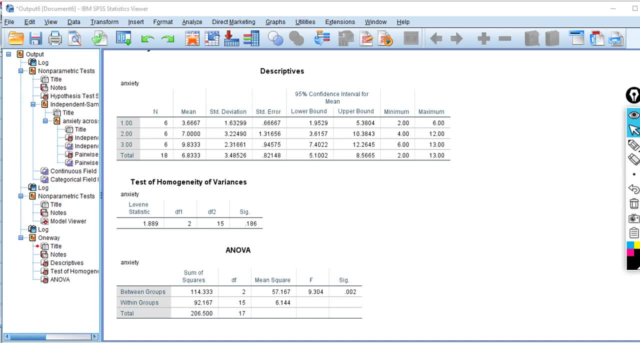 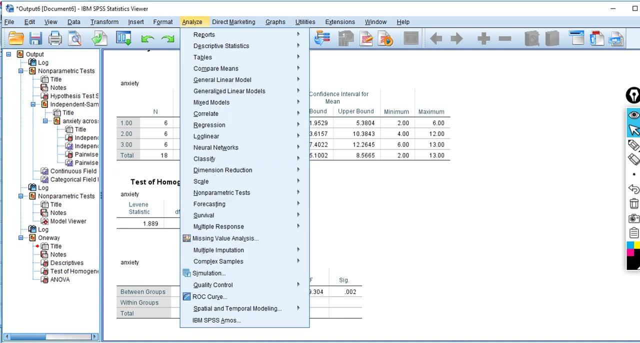 So that's the standard parametric one-way analysis of variance. Now let's run our analysis using the Kruskal-Wallis test. So to do this, we're going to go to analyze non-parametric tests, and there's actually two ways of running the tests. 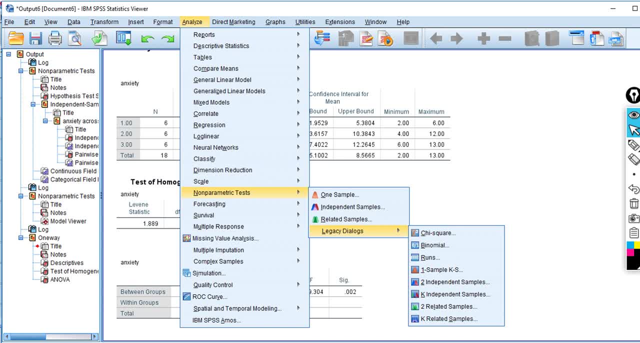 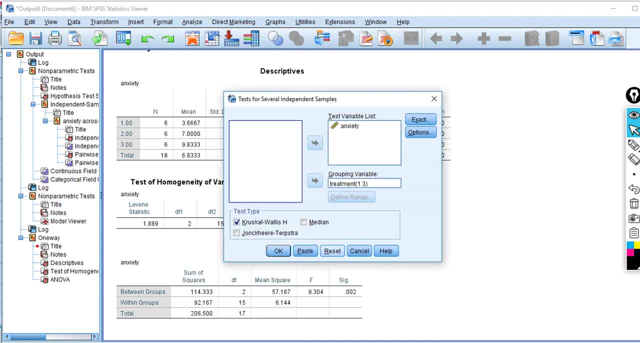 and what I'm going to do is I'm going to demonstrate both routes. so the first route we can go: through legacy dialogues, go down to K- independent samples- and click on it and I'm just going to reset it and show you we're going to move the. 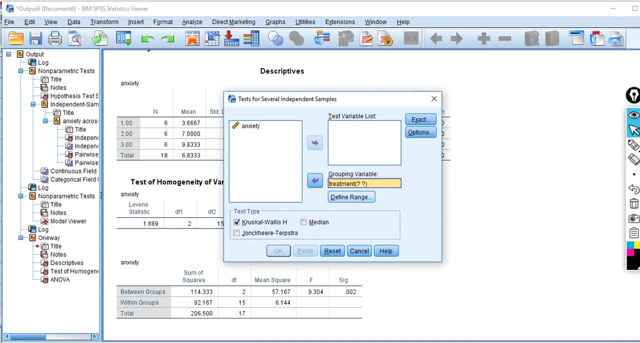 treatment variable over to the grouping variable box and, unlike the standard one way and oval, we actually have to define the range of values on our grouping variable. so I'm going to click on this button right here. and in our original data set, the the lowest value for our treatment variable is one, the highest. 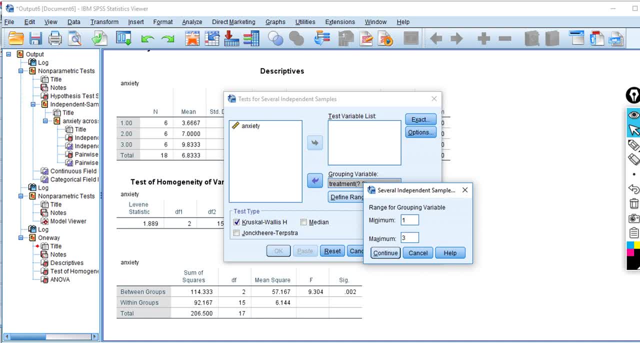 value is three, so that's going to be the maximum value. so we'll click on that. our type that in click on continue. so now you'll see that the range it is listed as one to three, then we'll move our dependent variable over to the test. 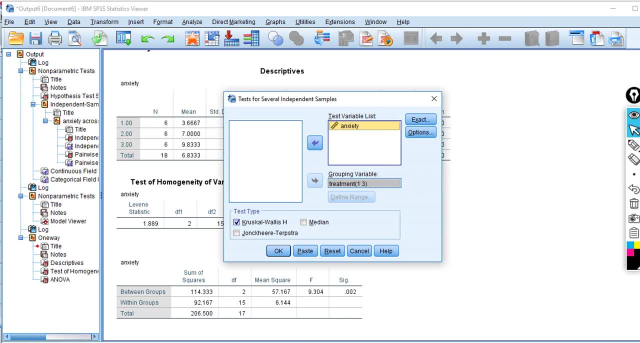 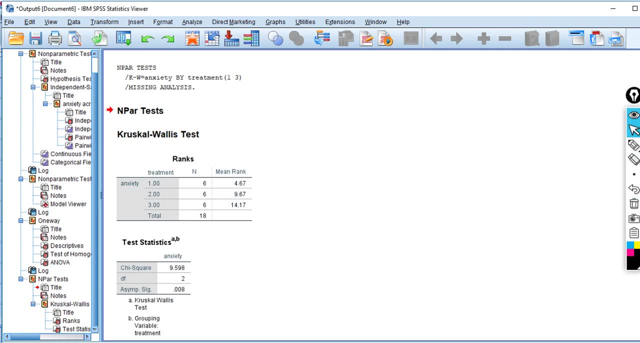 variables list box and the test type is set as Kruskal-Walsh right here. so now we'll click on OK and we get our output. so you'll notice that instead of getting the means on the dependent variable and basically where we were treating the dependent variable is continuous. you'll see that now we 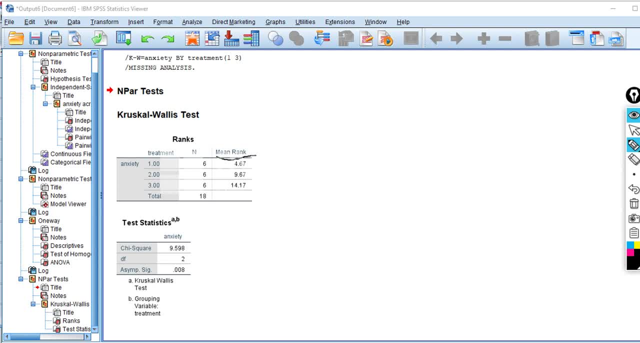 have mean rank. so, in other words, what happened is is that the program took the dependent variable and rank, ordered the values across the groups and then essentially computed the mean of the of the ranks within each of the groups. and there you go. so now you can see that the 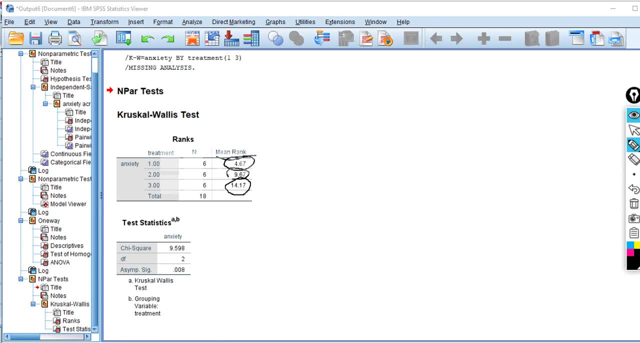 mean rank for group 1 was 4.67. the mean for a group two are: the mean rank for group 2 is 9.67. the mean rank for group 3 is 14.17. the test is essentially involving a chi-square test, so it's: this is a chi-square value and the degrees of 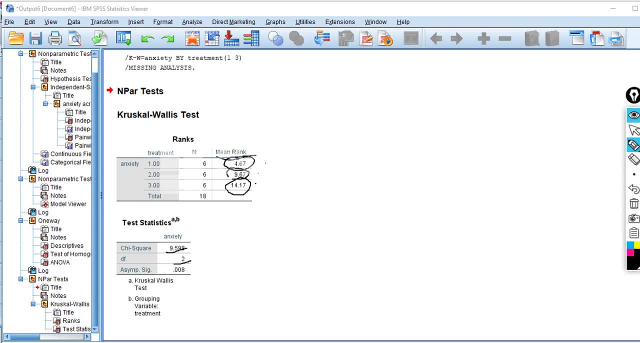 freedom, which is one less minus one, less the number of groups and the mean rank. And then we have the p-value that's printed out right here. So if we compare our p-value here, which is 0.008, against the conventional alpha level of 0.05,- 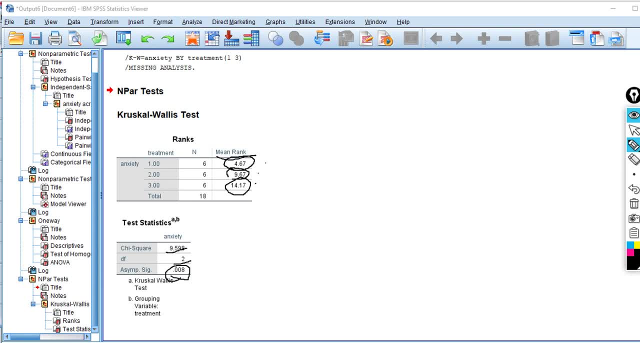 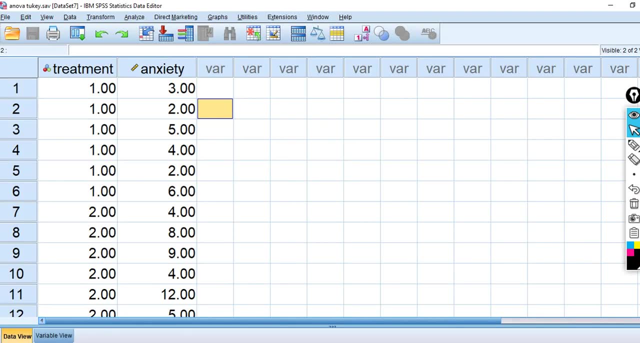 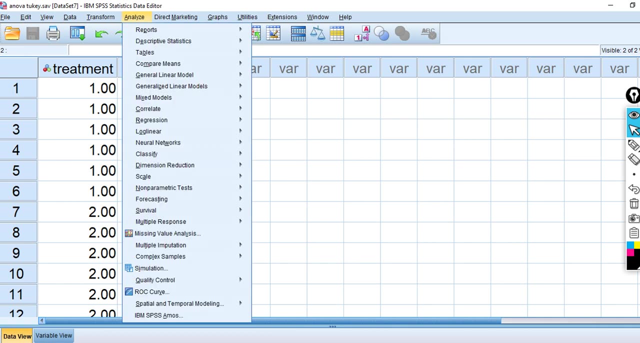 then we would reject the null and infer that there are differences across the groups on the dependent variable. So let's go back to the data set and I'll show you a little bit more details about how the process works. So what I'll do is just demonstrate it. 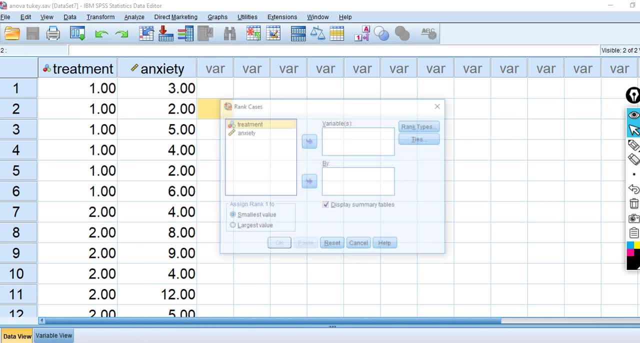 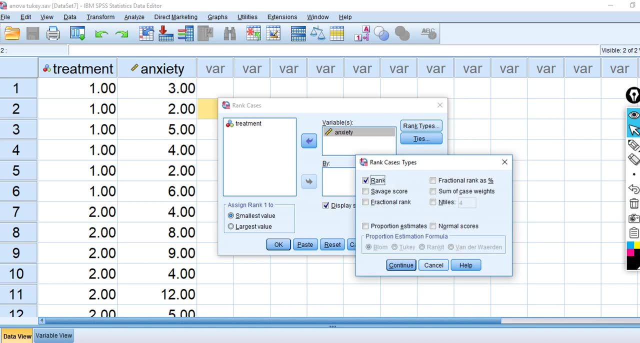 I'm going to go to transform and click on rank cases and I'm going to move the anxiety variable over to this box right here Under rank types. we just have it set at rank and then for ties we'll stick with the default for mean, right here. 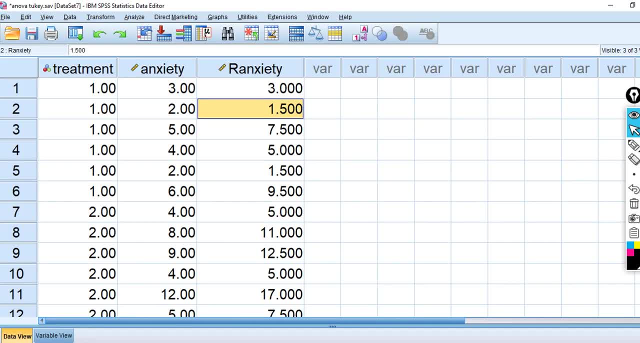 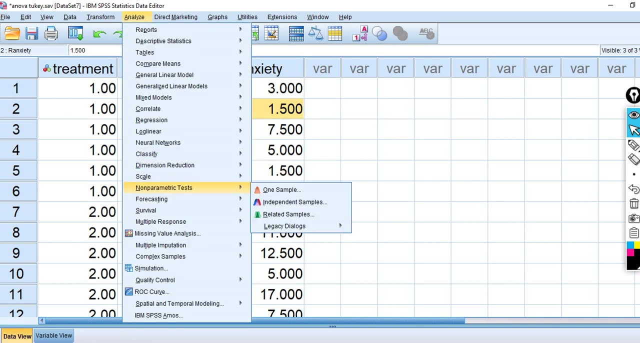 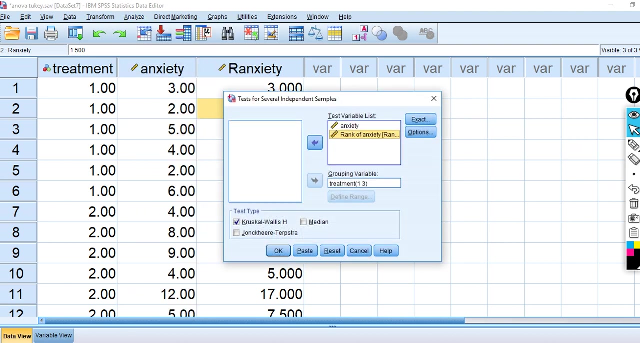 And then I'll click on OK. And so now you can see that the values on our dependent variable, the original dependent variable, have been assigned ranks across the groups. So that's essentially what's going on. And then if we were to run the same analysis on those ranks- in fact I will just move this over here so we can have a point of comparison- 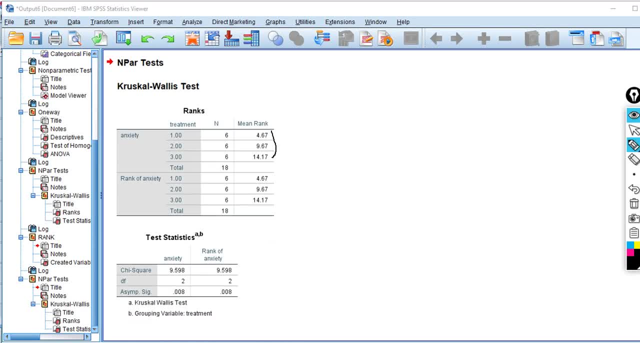 you'll notice, in this case, the mean ranks with respect to the original variable are going to be exactly the same as for our rank variables. So you can see, that's the same: The chi-square value, the degrees of freedom, everything is exactly the same as before. 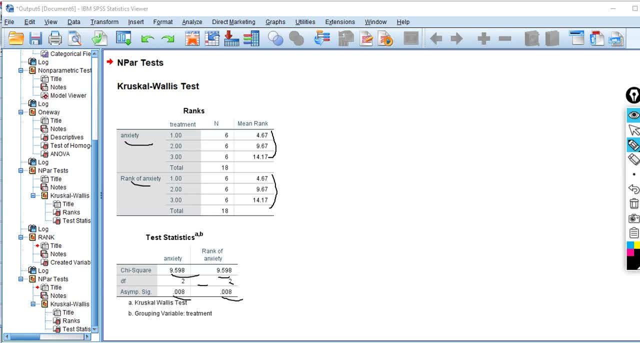 So that's what I was meaning when I was. I was saying that the Kruskal-Wallis test is essentially comparing the mean ranks between the groups. So what that also means, then, is that your original dependent variable can be continuous, or it can be in the form of ranks, basically an ordinal variable. 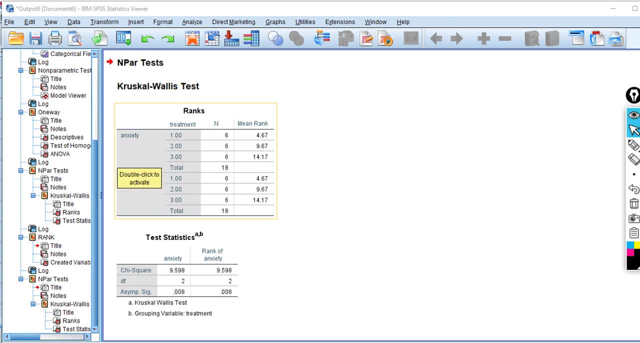 If your original variable is continuous, then essentially the program will convert that variable to ranks and then compute the mean ranks, Whereas if your original variable is actually already in the form of ranks, then you'll get the same thing. So you're essentially comparing the groups in terms of ranks. 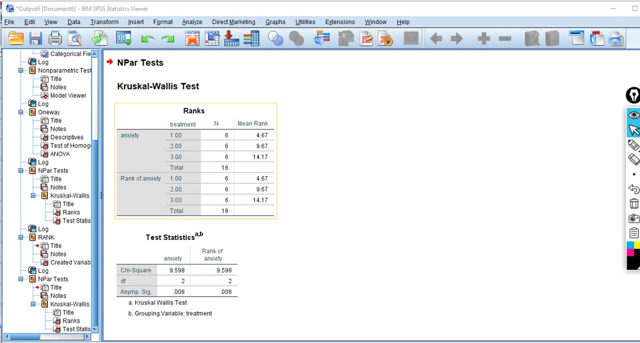 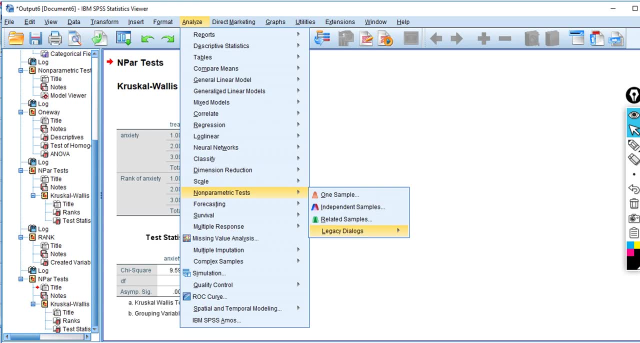 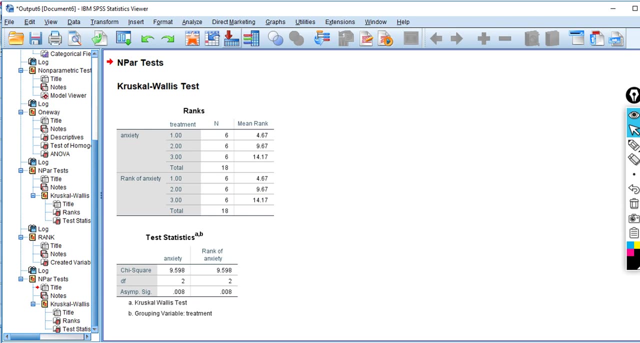 Now, if you wanted to follow up and test for mean differences, you could do the Mann-Whitney test kind of manually through the program, just by using the two independent samples and then carrying out pairwise differences there, Or a better option is actually. 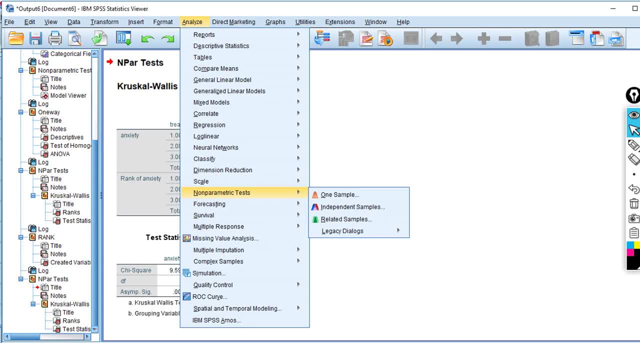 to use a different approach, where you can ask for pairwise differences at the same time that you're carrying out the standard Kruskal-Wallis test. So to do this, I'm just going to go to non-parametric tests, go to independent samples, right here. 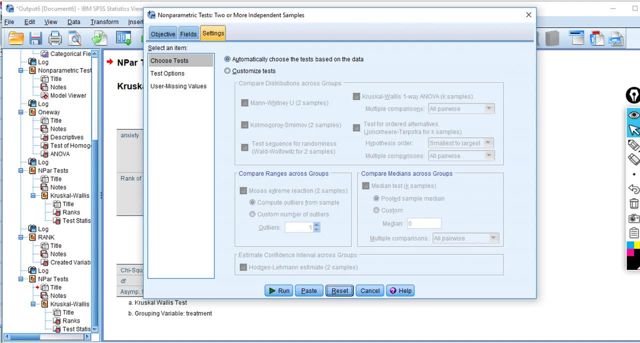 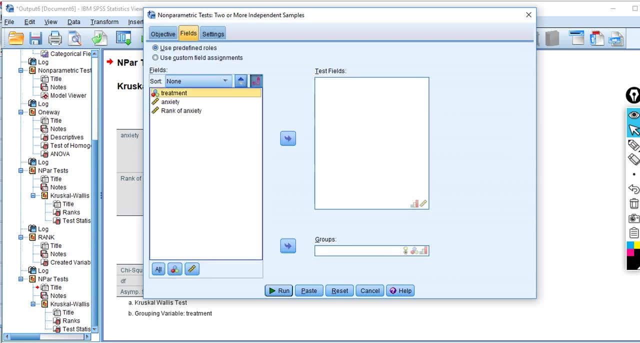 And I'm just going to reset this and walk you through. So now you'll see that, under objective, we're going to leave this as it is. Under fields, we're going to move our independent variable over to the groups box and our dependent variable anxiety- over to the test. 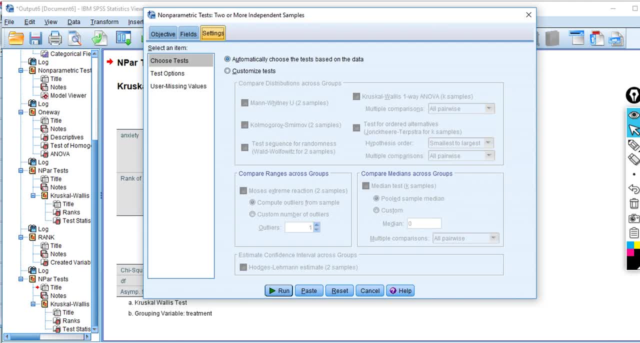 So we're going to go to the test fields box, Then we'll click on settings and then click on customize tests And you'll notice that if we had just two groups and we wanted to perform the Mann-Whitney through this, we could just click on that. 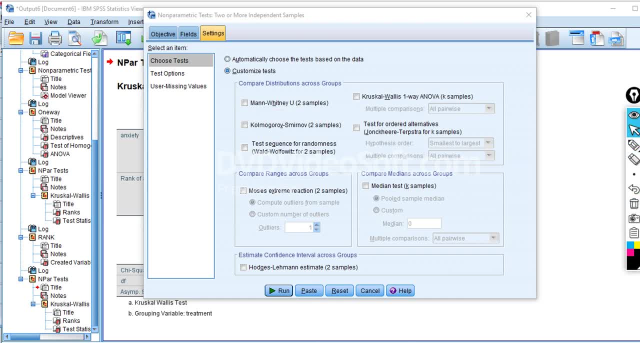 But instead we have three groups and I want to carry out essentially the non-parametric ANOVA as well as ask for pairwise comparisons. So I'm going to click on this box right here And you'll see that where it says multiple comparisons, all pairwise. 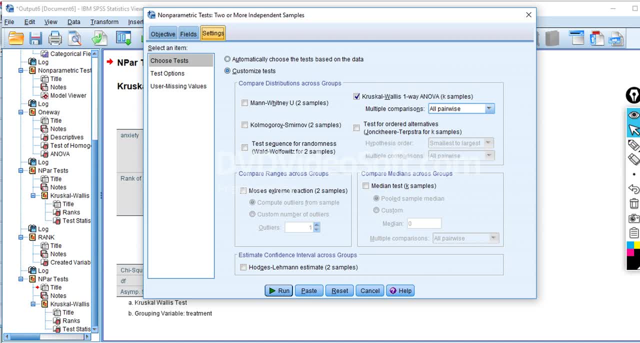 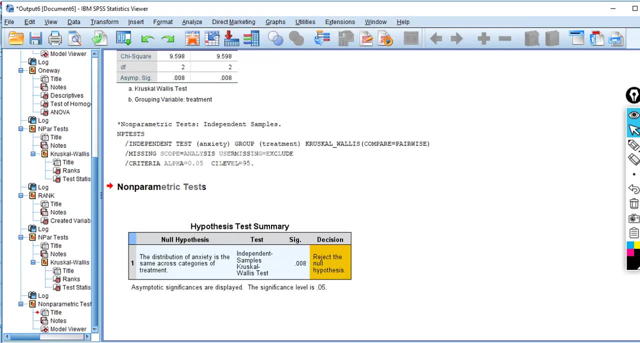 And so in this particular case, I'm just going to leave that as it is. Then I'm going to click on run And you'll see that we get this little box down here- Hypothesis test summary- with the P-value that's printed out right here. 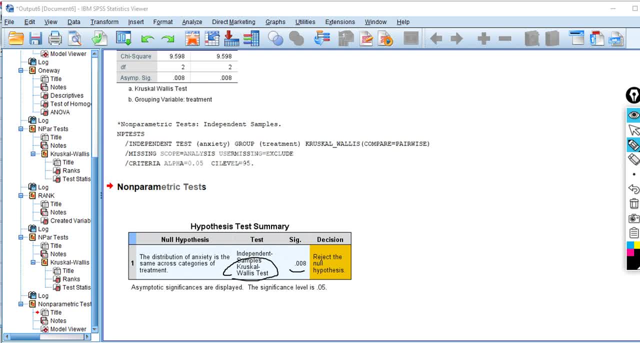 And so you can see, it says Kruskal-Wallis test And they actually, under this particular menu system, it gives you a decision basically rejecting the null hypothesis at the 0.05 level. So in other words, we would infer that there are differences between the groups. 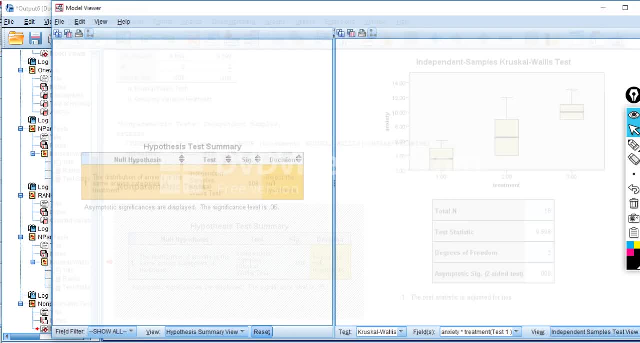 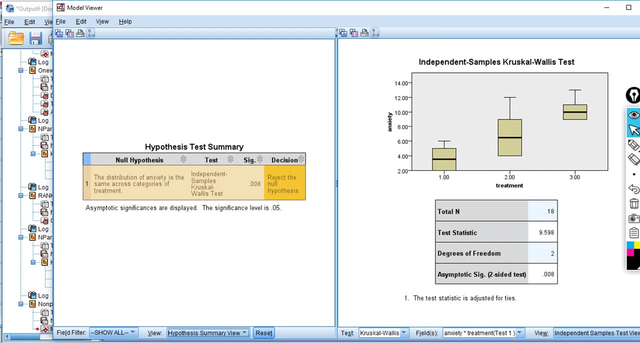 on the dependent variable. So I'm going to double-click on this. If I want a little bit more detail, you can go under this model viewer right here And you have different options that are available to you- little drop-downs below. 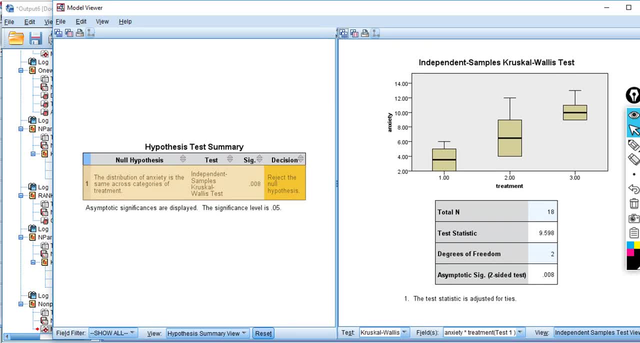 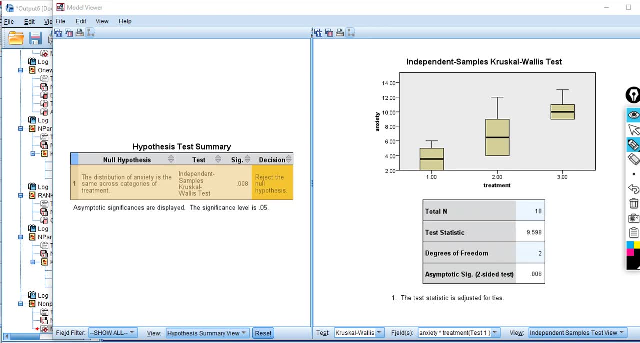 But you can see we've already rejected the null hypothesis for the one-way non-parametric ANOVA. And then over here you can see that we get essentially a plot with, you know, kind of a box plot, if you will. 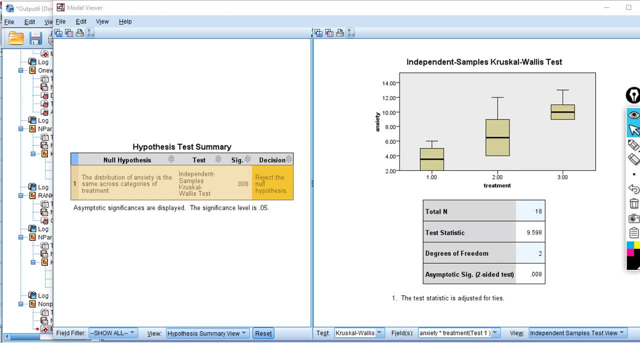 And what we'll do at this point, though, is you'll notice that we have the total N- This is the chi-square value that I'd shown you before- and the degrees of freedom, and then the asymptotic significance level. So all of this information, if you wanted this, when you're writing up your results. 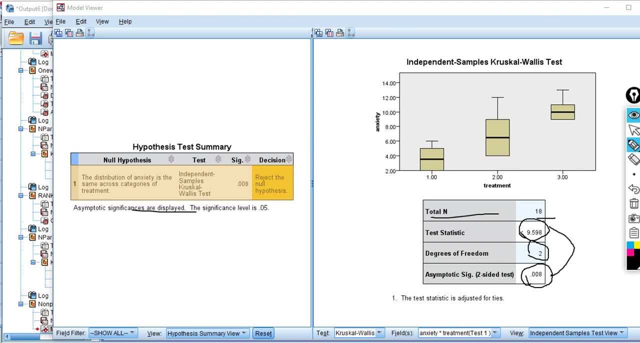 this box right here is not going to give all that to you, But if you want to report on the chi-square value, degrees of freedom and P-value, you have it right over here. Then down below you can see it says: test is Kruskal-Wallis. 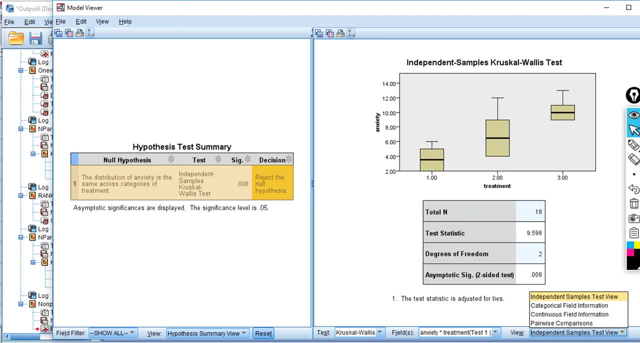 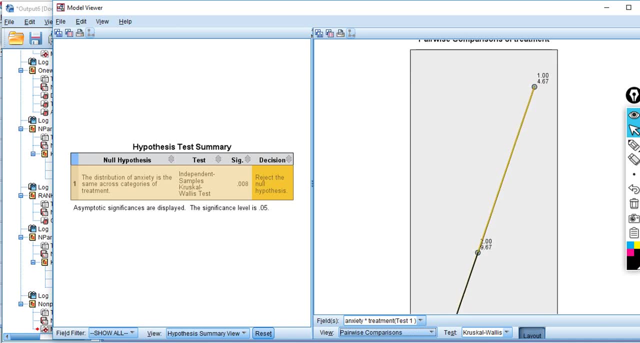 And then, if I want to get pairwise comparisons, I can click right here This little drop-down and then click on pairwise comparisons and this is what it's going to look like. So you can see, as I scroll, what you get. you can see that we have group one right here. 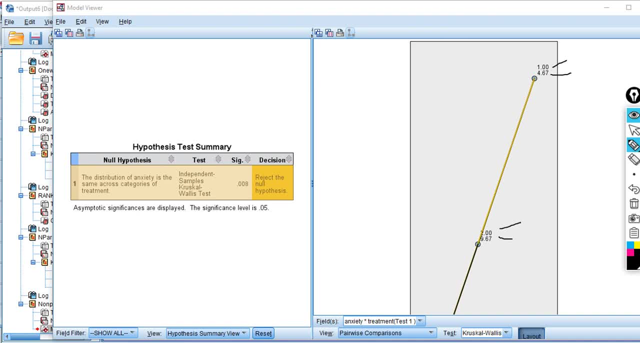 and this is the mean rank. group two, mean rank. And then, as we kind of scroll down a little bit further, we get group three And the mean rank here And then, if I want the actual pairwise significance test, these are just basically Mann-Whitney tests. 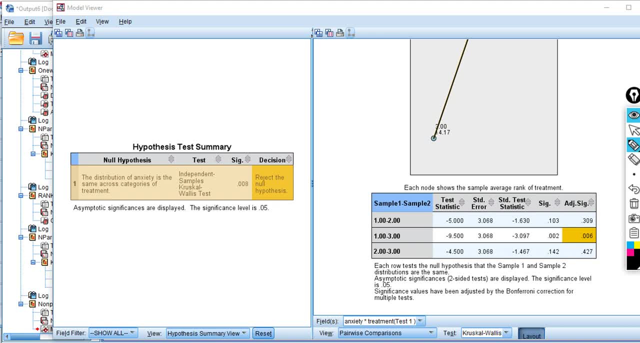 So you can see that I get the test statistic right here as well as the P-values for significance, and then there's sort of an adjusted significance right here, And the adjusted significance are basically involving a correction, basically a Bonferroni correction. 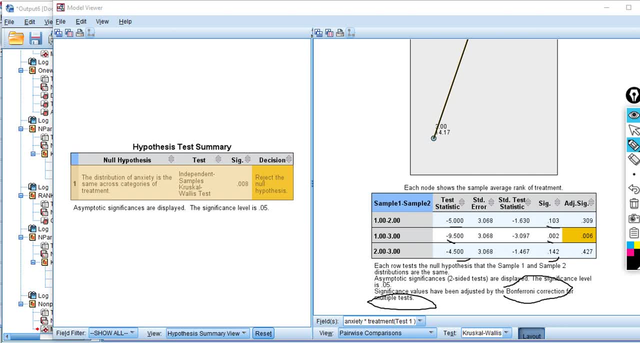 So if you want to adjust the P-value- the P-values for the fact that you're carrying out multiple tests- then you can just click right here. Then you can just use these P-values and report on those. as opposed to this, These significance levels are not being adjusted for the multiple tests. 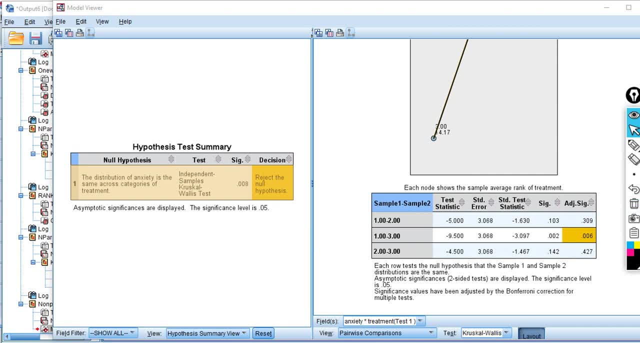 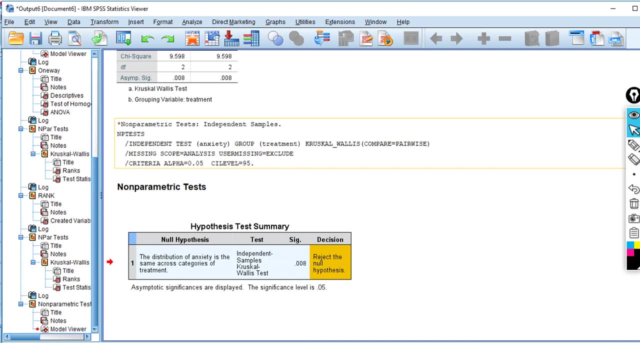 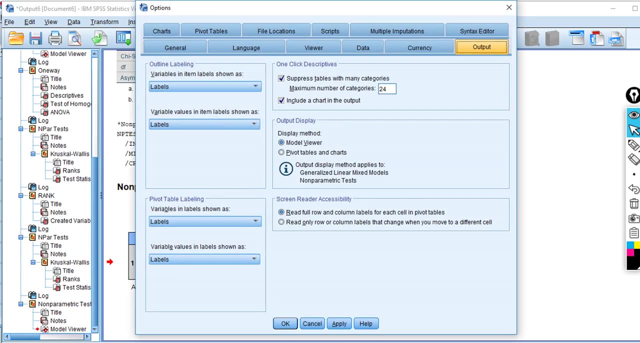 that are being carried out. So, at any rate, that's using sort of the model viewer approach. Now there is another way in which you can get the output, and if you go under edit and options, click on output, you'll notice that this is using the model viewer display method. 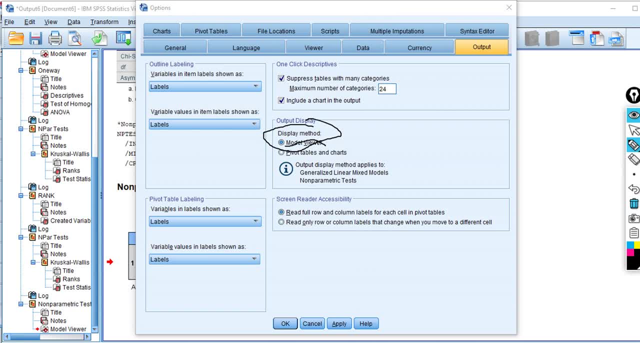 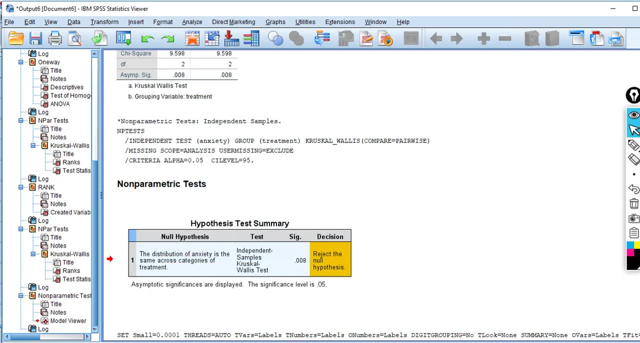 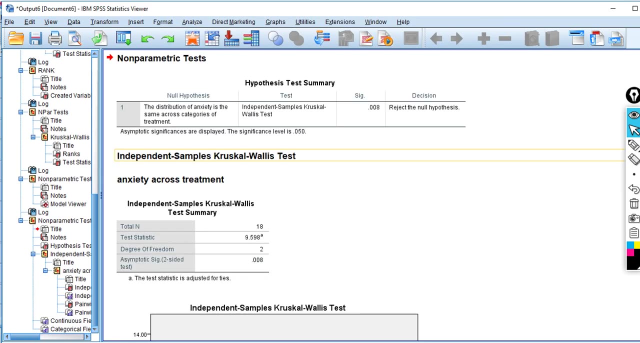 It's a little bit hard to read right there, but there it is. If you want your output in a little bit more standard format, we can click on pivot tables and charts, and when we click on okay and then run our analysis, our output is a little bit more conventional. 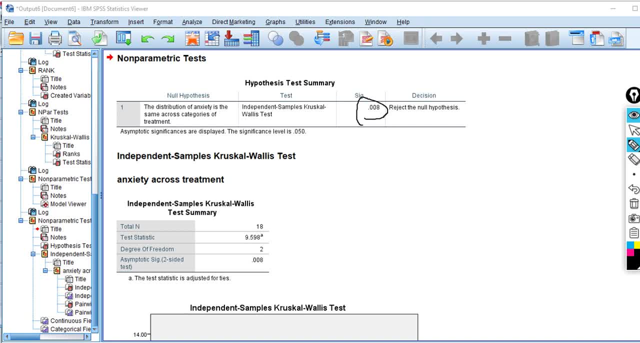 So you can see there's the P-value right here, and then that's the same value that we have down here, as well as the test statistic degrees of freedom and so forth, And then as we scroll down you can see we have little box plots here. 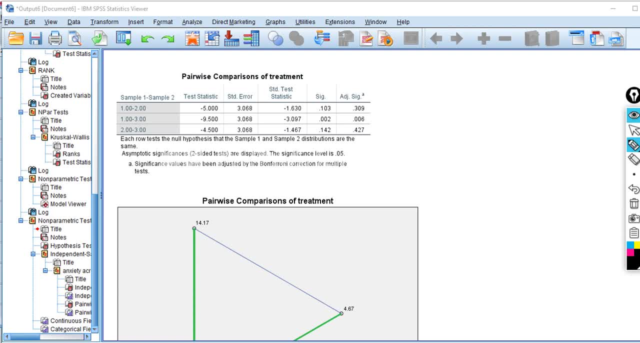 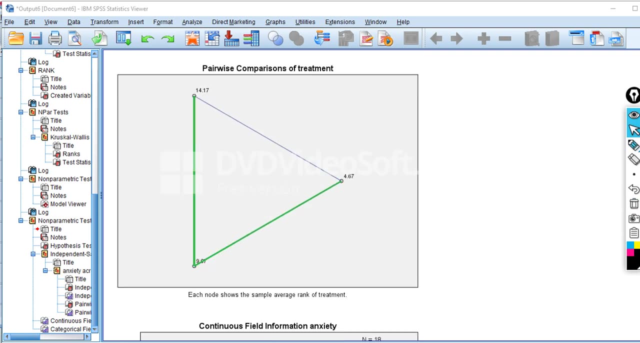 and then you can see that we get the same test statistics that we had before: the P-values, the significance levels and then the adjusted significance levels involving the Bonferroni correction that you have right there, And then, if you want, the mean ranks for each of the groups.